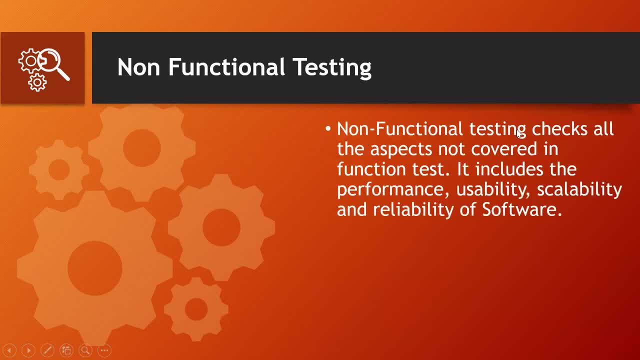 So non-functional testing checks all the aspects not covered in functional test. It includes the performance, usability, scalability and reliability of the software. So the performance is what exactly? speed, stability, stability. So the performance is what exactly? speed, stability, stability. 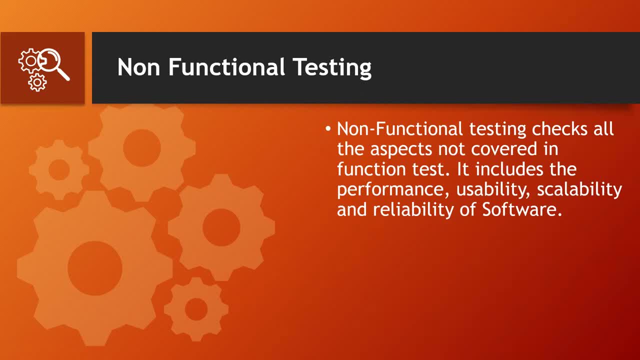 speed is what it determines whether the application responds quickly. we have seen usability is what, whether the application is user friendly. You have seen it's an user friendly Flipkart. scalability is what determines maximum user moves. This is a problem the software application can handle. that is, with the scalability and reliability is what the software should be working as. 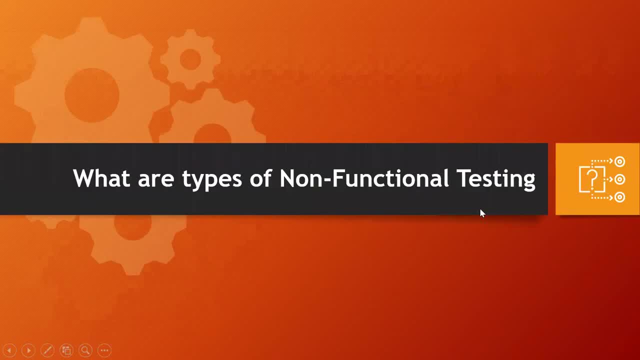 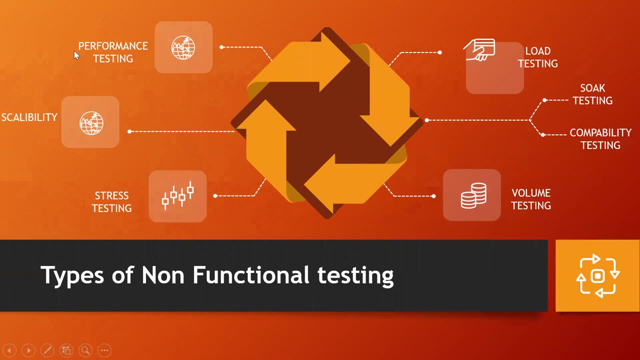 for the expectation for long duration Of fter knowing why and what. now let's see what are the types of non-functional testing. so performance testing, load testing, soak testing, comparability testing, volume testing, stress percent, scalability testing. so these are all the types of the non-functional testing. 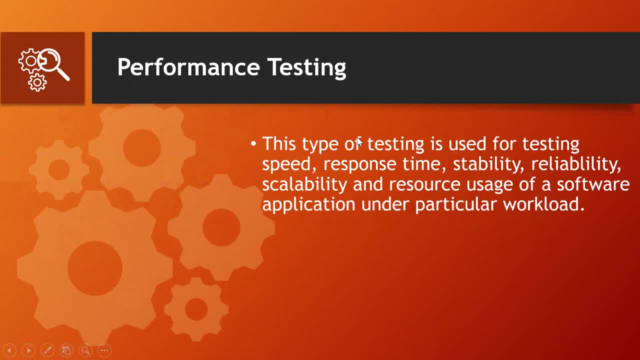 let's see one by one. so testing in detail now performance testing is what this type of testing is used for. testing speed: we have seen the speed response time after clicking something, how much response time it's getting to place an order, how much time it will require. that is for the 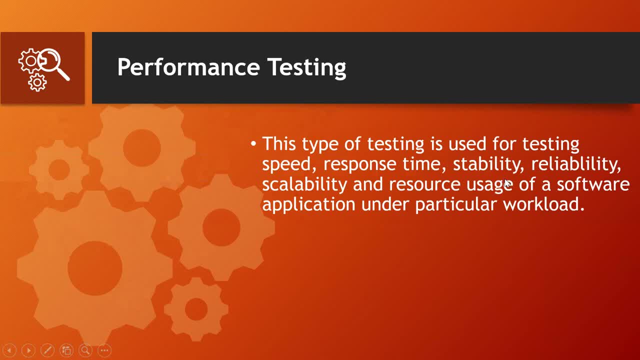 response time stability. it's checking the stability: whether the load isn't very, whether it's the application is stable or not. reliability for long run- is it working or not? scalability and resource usage of a software application under particular workload. now in this, what happened? user and response. 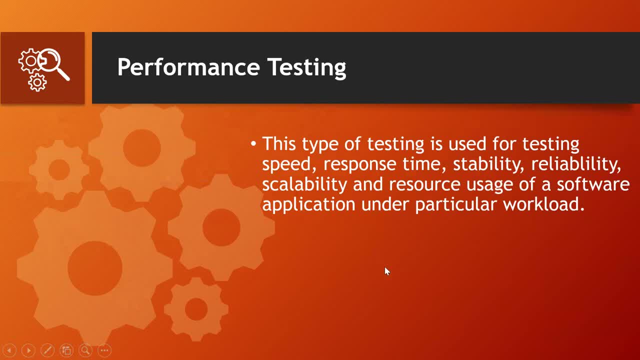 time. there are the two categories on that we apply the load. let's take an example: flipkartcom. its requirement is nearby to 10 lakh. user should log in and the response type should be two. second now the load is what? 10 lakh is a load? 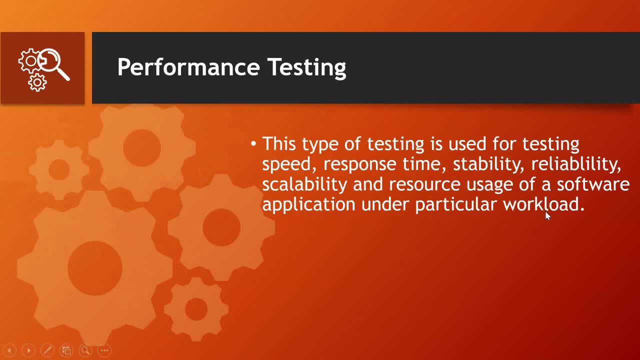 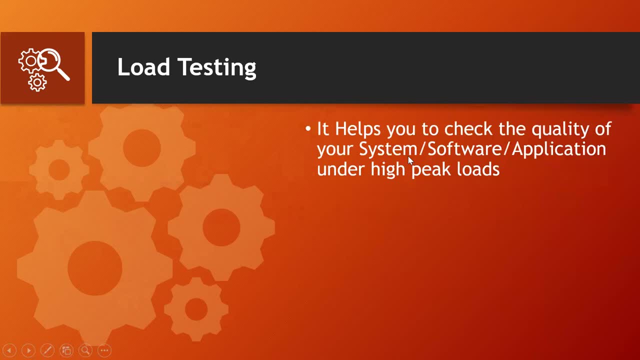 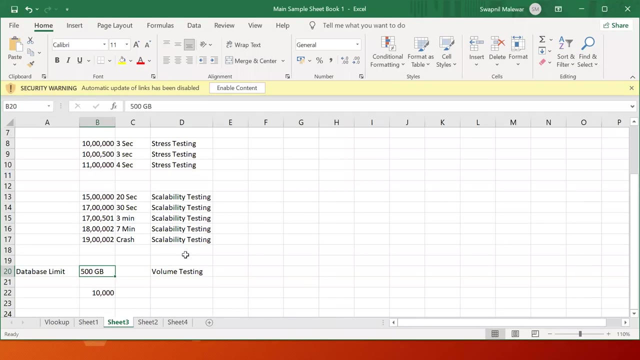 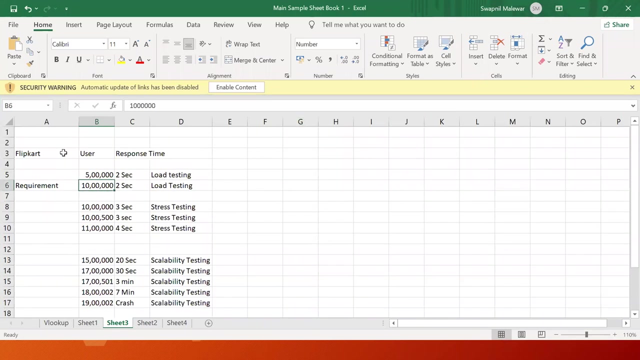 okay, it's an user load. that is where the particular workload they are see. after that, let's see the load testing. it helps you to check the quality of your system software application under high peak loads. let's understand this by one example. okay, now here the requirement from the 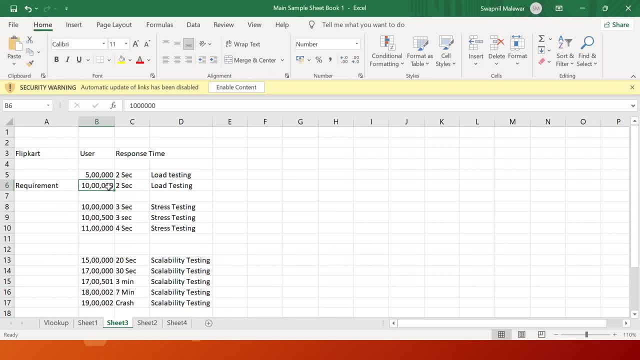 flipkart is what that tan like user should be able to log in at one time and the response time should be two seconds. so in load testing, what we will be checking, we will be checking this condition as well as the condition which is less than the current. 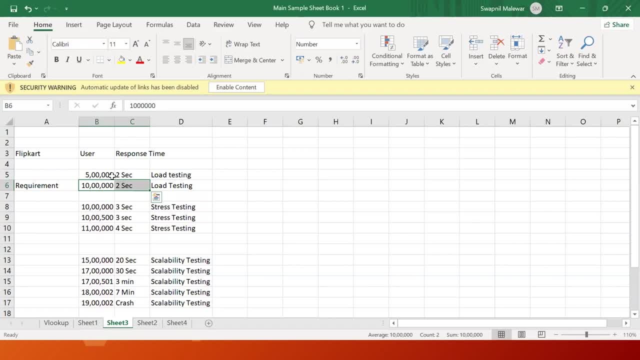 requirement, that is, 5 lakh. you. we check whether what is the response time. is it the two seconds? it is the one second. whatever it is, then what is the response time for the seven lakh user if at once they're log in? so we check in the load testing. 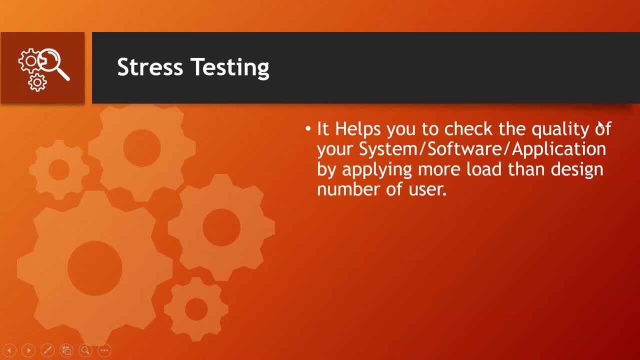 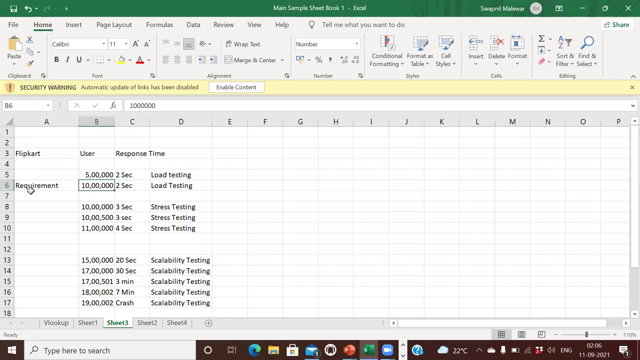 load testing. let's see stress testing. it helps you to check the quality of your system application by applying more load than the design number of the user. okay, let's understand this now. the design user requirement from the flipkart is 10 lakh and the response time should be. 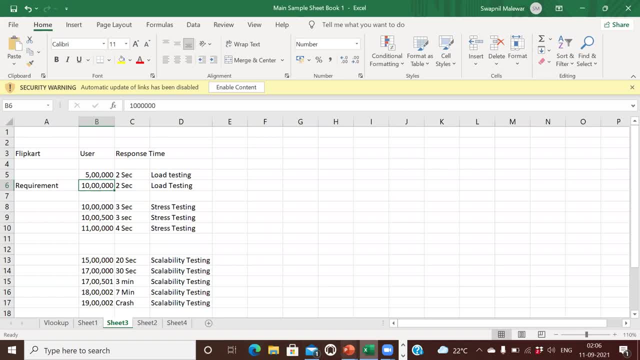 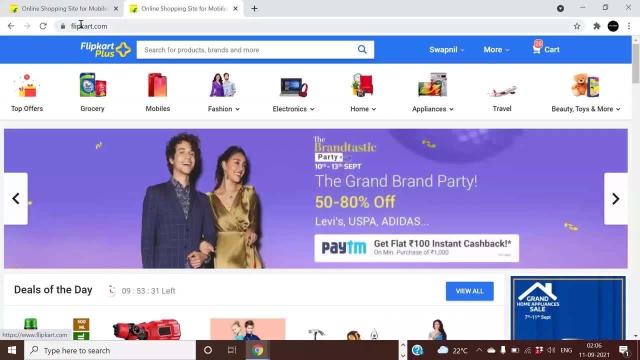 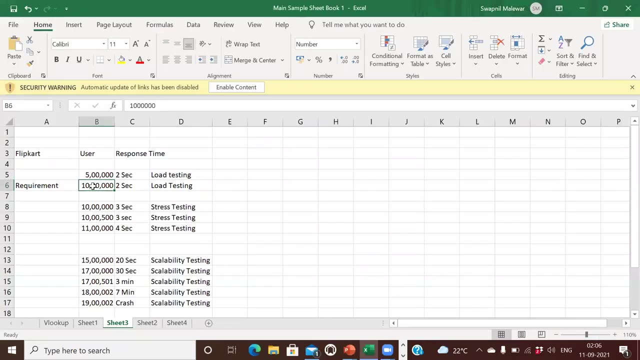 two seconds response times is what again? i will show you if i am entering flipkartcom that it should not go beyond two seconds. it should be on before two second. that is the response time. now in stress testing is what like after 10 lakh user, we check whether the response time is two. 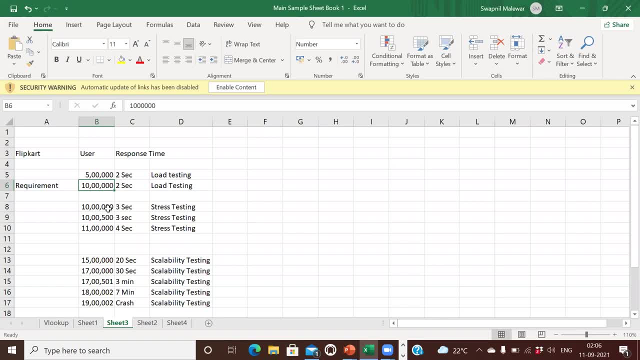 seconds. no, after 10 lakh user, the response time is coming three seconds after 10 lakh 500 user. again, this is the three second. after that we are increasing the user 11 lakh. it's giving four second time to open the web console or the flipkart. 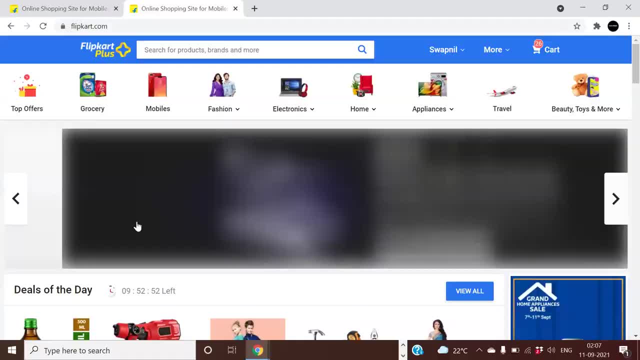 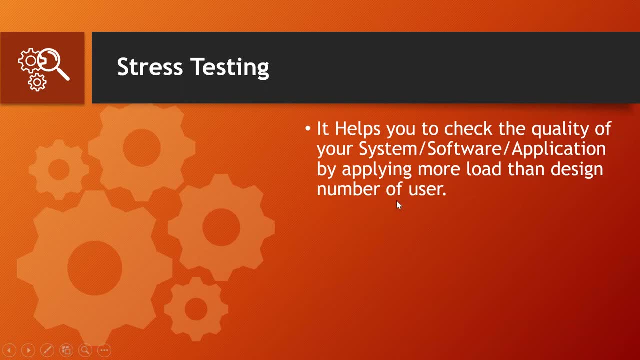 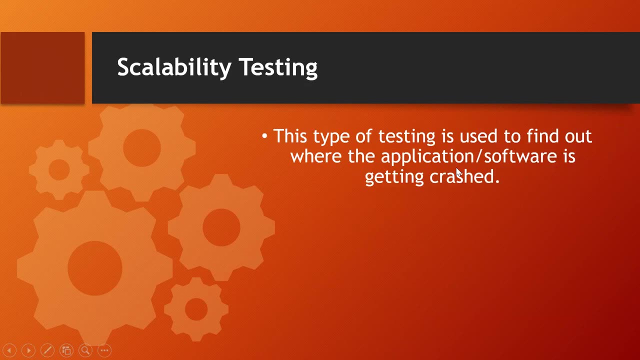 website. so this is all about the stress testing: applying more load than the design number of user. that is stress testing. scalability testing is what this type of testing is used to find out whether the application software is getting crashed. now, every software gets crash at certain time, so at what time it get crash, that is tested in this testing. 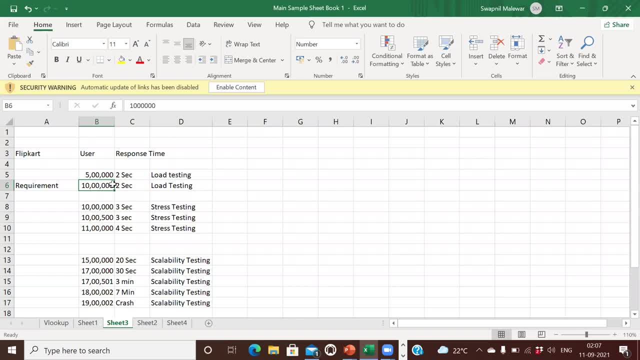 let's take an example now. the requirement was 10 lakh users- two seconds. in the scalability testing we are increasing the user. that is 15 lakh now. it's taking 20 seconds. for the 10 second: it's taking two seconds. for the 15 lakh: it's taking 20 seconds. 17 lakh: it's taking 30 seconds. 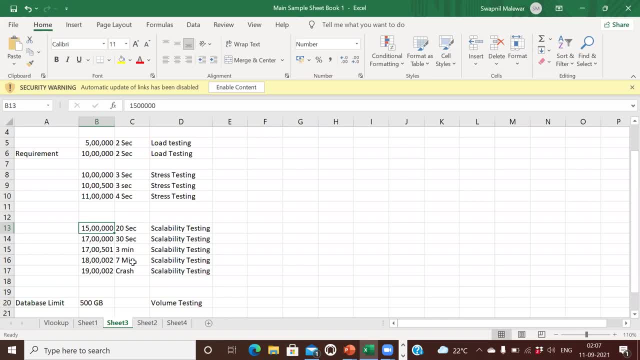 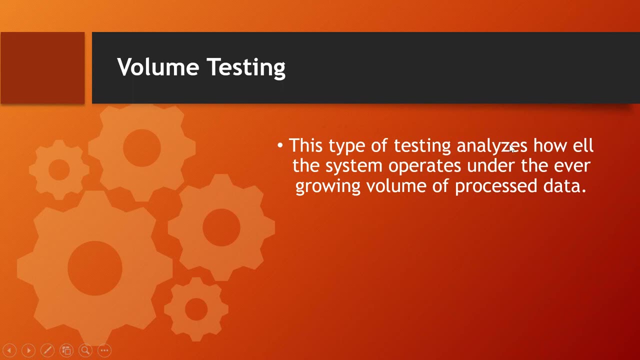 17 lakh 500 and one- it's taking three minutes. 18 lakh- it's taking nearby to seven minutes and at the point of 19 lakh it get crash. that is what the work of the scalability testing is. after that volume testing, this type of testing analyze how, how well, the system operates under the 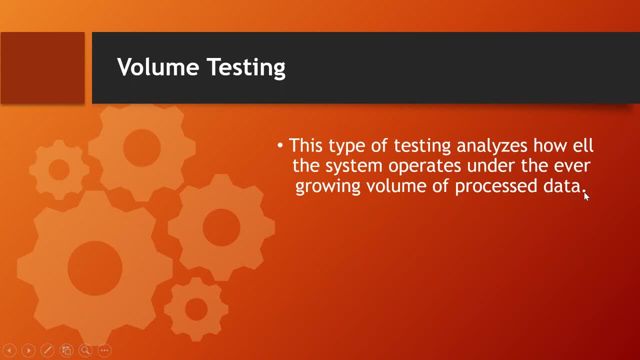 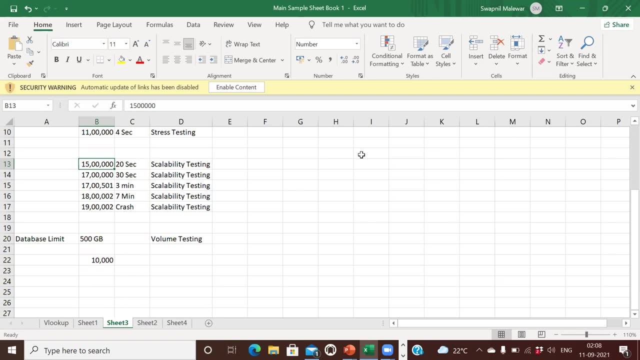 ever growing volumes of the process data. the process data is what. let's take an example of: the flip card. flip card is having huge kind of a information available on its website. so there are some of the products now. there are the information about the user: someone has to buy, sell, whatever it is. 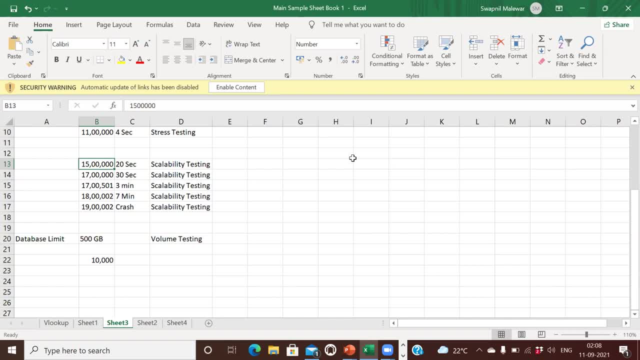 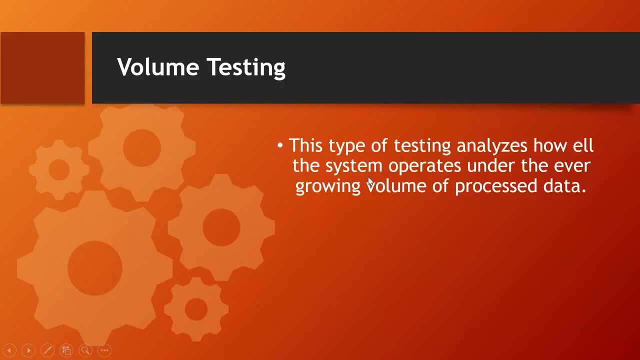 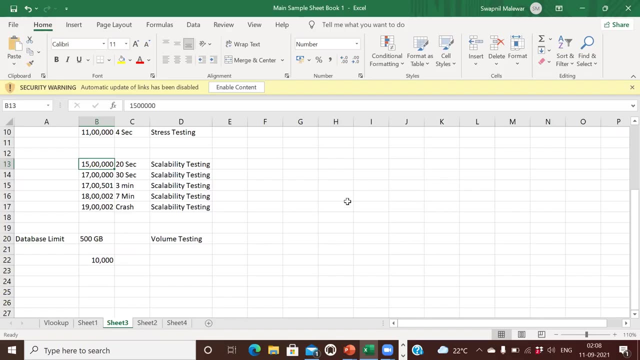 okay now, flipkart had given the daily limit of 500 gb data. so in the volume testing we check whether all the data, whether all the data or under the growing volume of the process data, the process data which we are having on the flipkart website, whether it's getting tested. 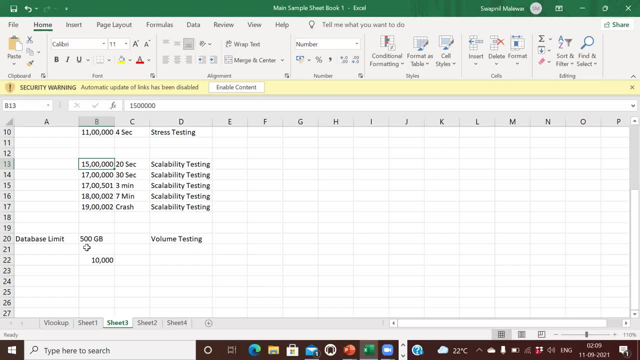 till 500 gb if the data is getting beyond 500 gb, so how the system is reacting towards it, whether it's getting crash or not, that is what we check in the volume testing. but with respect to data, okay, after that, soak testing, this type of testing. 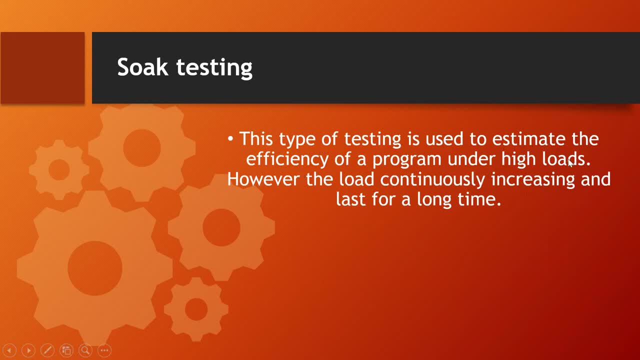 is used to estimate that the efficiency of a program under high loads, however, the load continuously increasing and lasts for the long time. best example for this we can say: let's say previously we were having tv, okay, now in this tv by accidentally. or we can say, while watching you were sleeping, so for 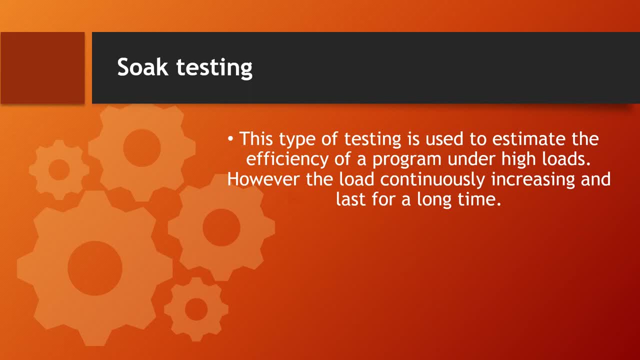 12, 10 hours, whether the tv is continuously working or not, it was working. so that is what soak testing is. that is for the non-technical aspect. now let's see for the technical aspect of software. now this software currently is about microsoft office. we are using powerpoint. 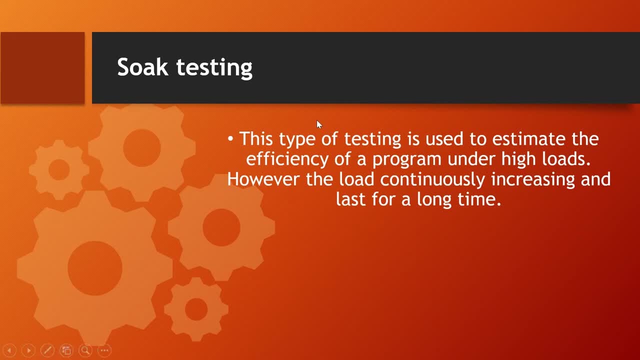 so what they have done in the soak testing, so they have checked whether the ppt or this slide or any slide can continuously work, like one hour, it will work. two hours, it will work, three hours, it will work, then four hours also, it will work. what about five, six, seven, what about more than ten? 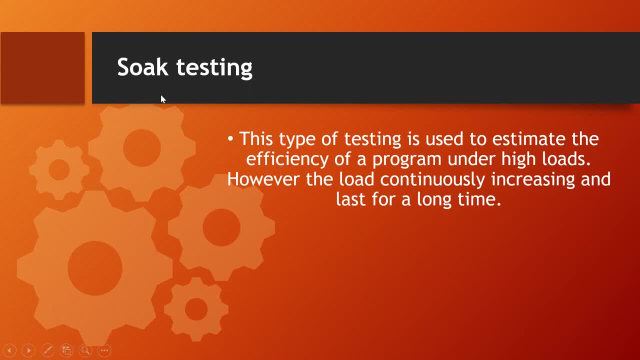 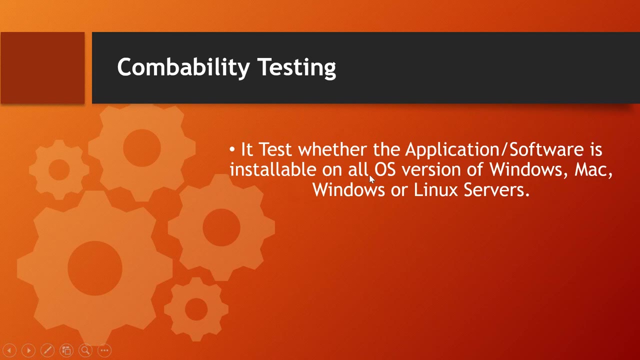 what about two to three weeks? will it work? so this is all about smoke testing. it is also called as endurance testing. after that, the last one is compatibility testing. it tests whether the application software is installable on all os version of windows, mac windows or linux server. let's take an example. 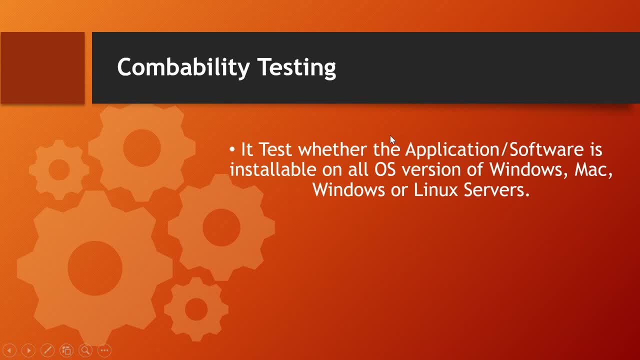 now we can say that microsoft office is designed for windows windows version. okay, now can we install the microsoft office on windows server or linux server? it's not possible. it's very hard to use. okay, that is what compatibility testing is. okay. so this is what non-functional testing was: why, what and what are the types, if you have any? 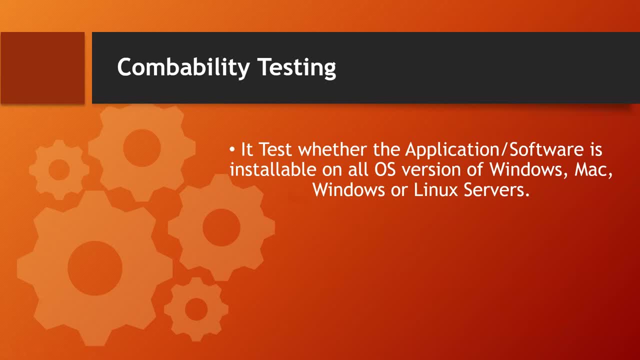 kind of a doubt, do comment. we will definitely do our best to provide you solution for your question. thank you.